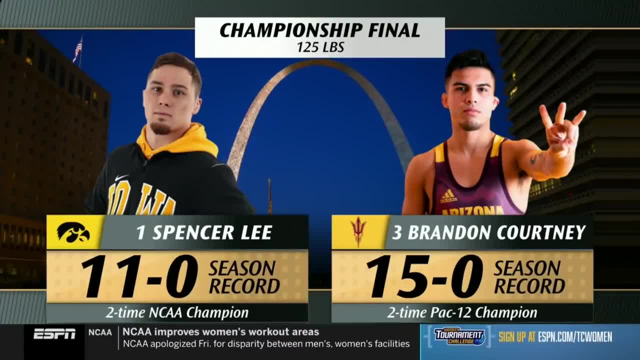 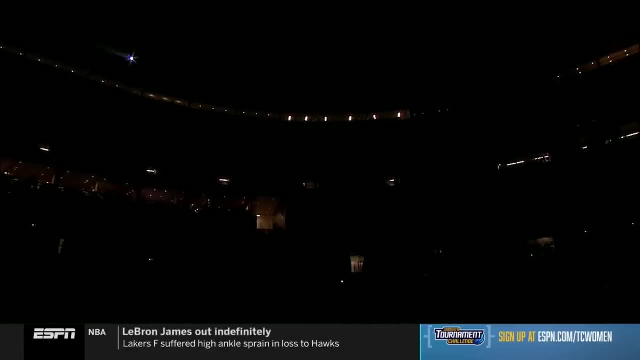 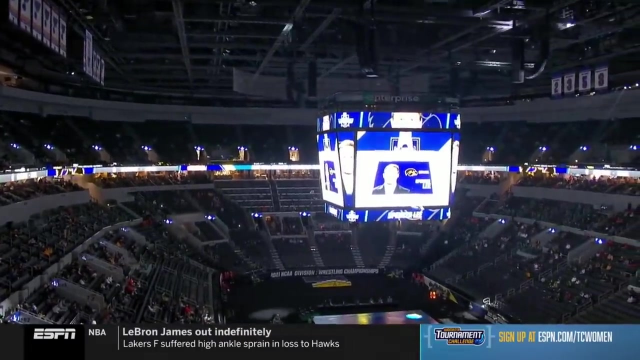 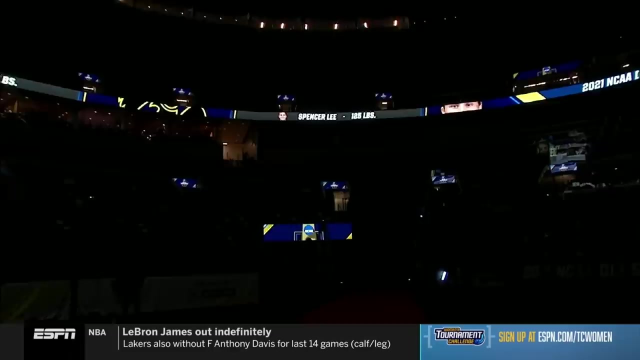 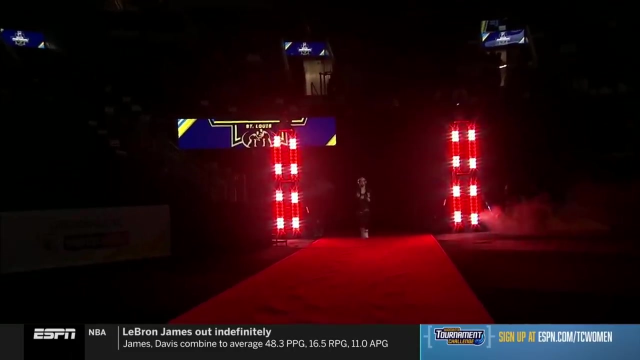 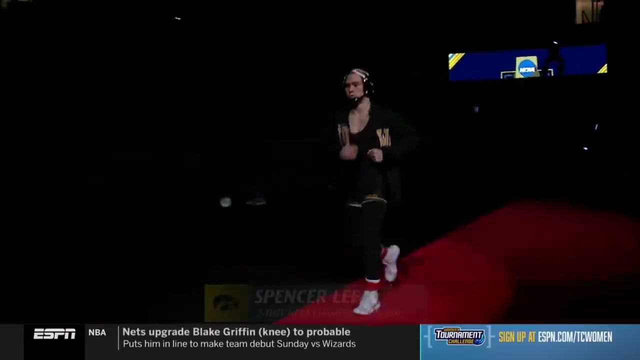 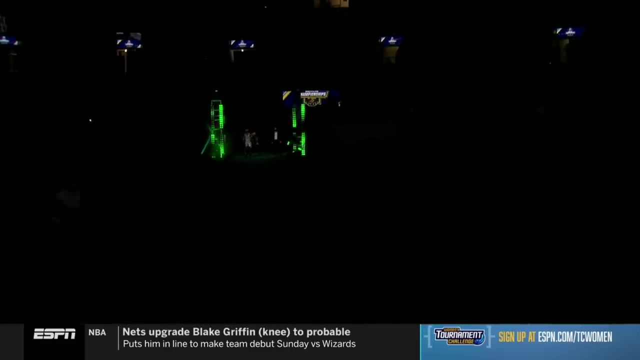 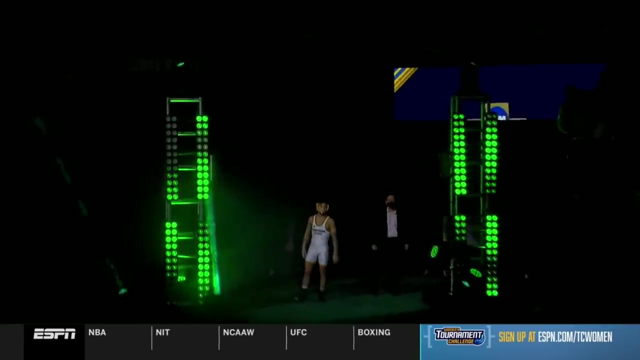 pluscom Spencer Lee going for his third NCAA championship against two-time Pac-12 champ Brandon Courtney of Arizona State. Wrestling for the championship at 125 pounds. Wearing the red from Iowa, Spencer Lee And his opponent wearing the green. 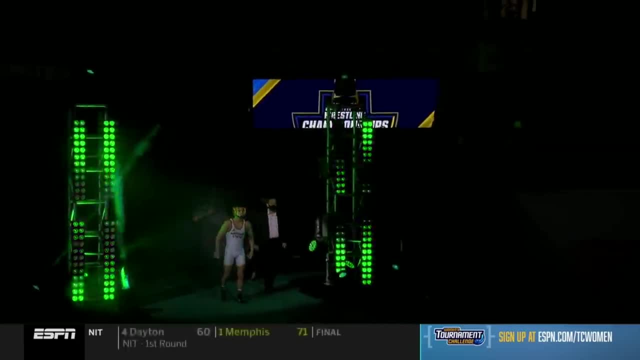 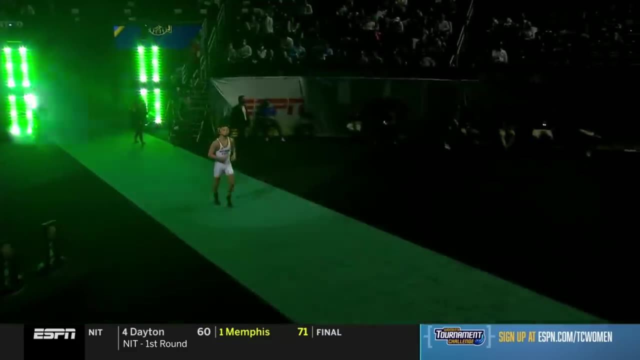 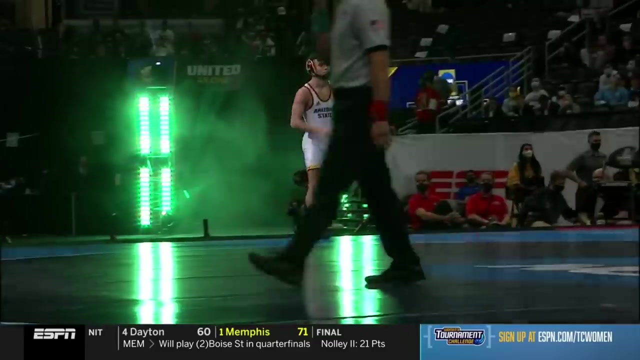 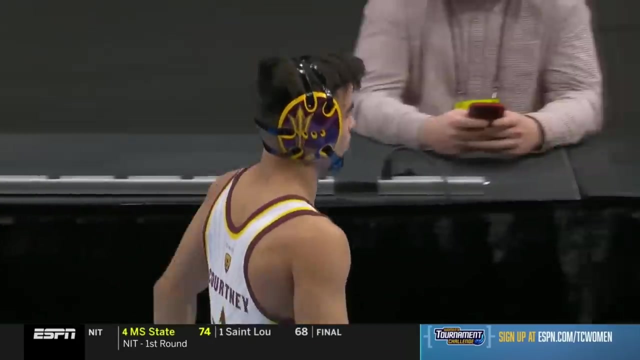 representing Arizona State. Brandon Courtney 2011 at 125 for Arizona State was pretty special. Our buddy, Anthony Robles, a champion that year in Philadelphia. However, it is a big mountain to climb here to try and stop Spencer Lee. He's outscored the opposition. 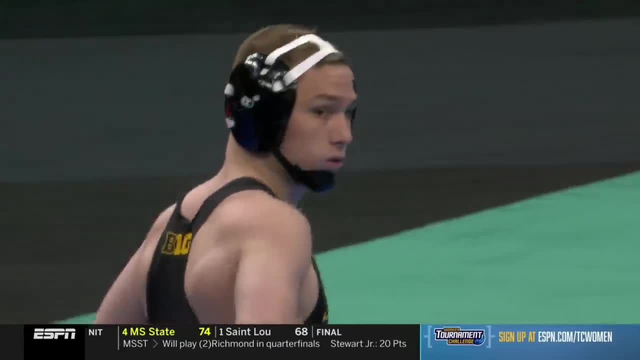 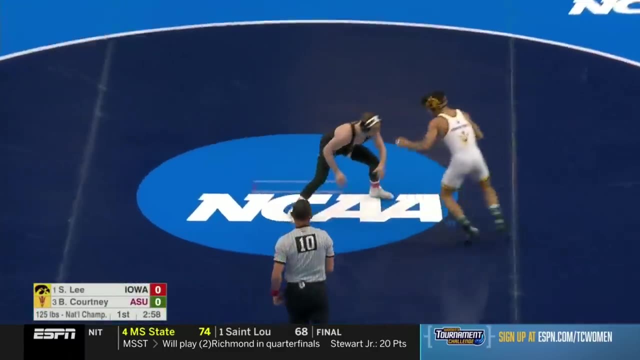 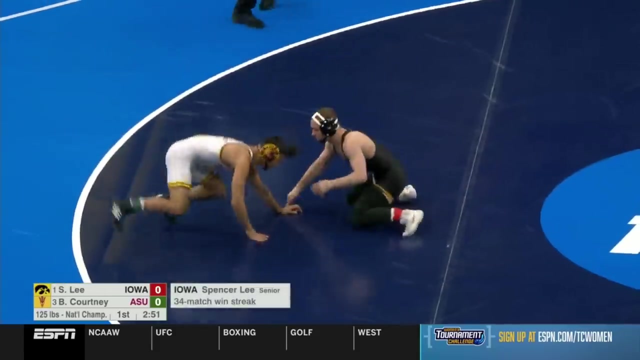 He's outscored the opposition here in St Louis 52-8, and is trying to become the seventh three-time champion in Iowa's history. Spencer Lee, two-time junior world champion, cadet world champion out of Franklin Regional. 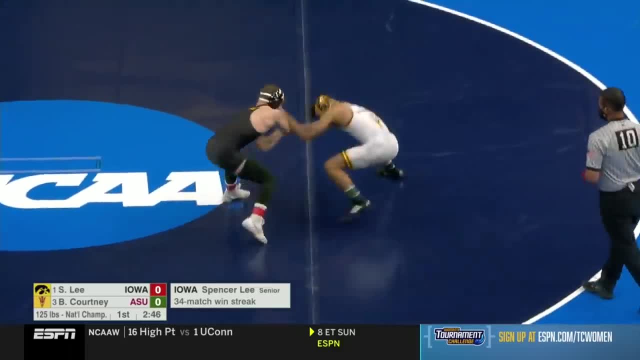 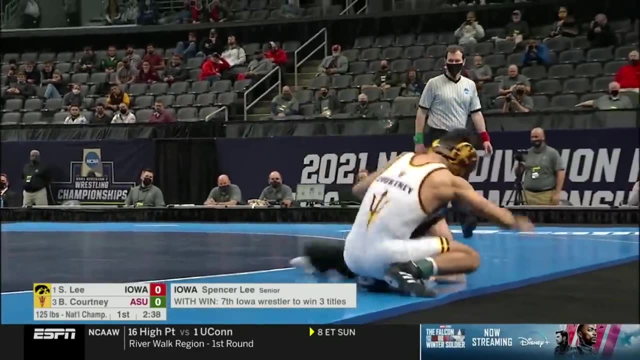 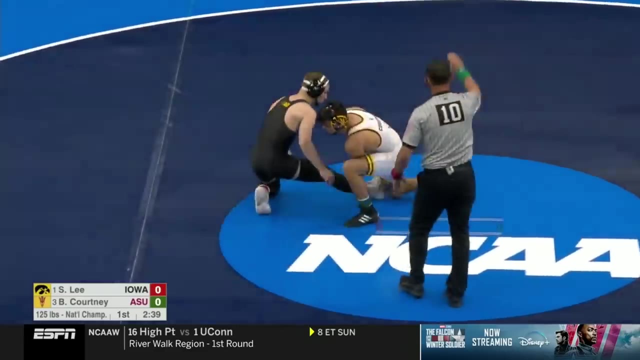 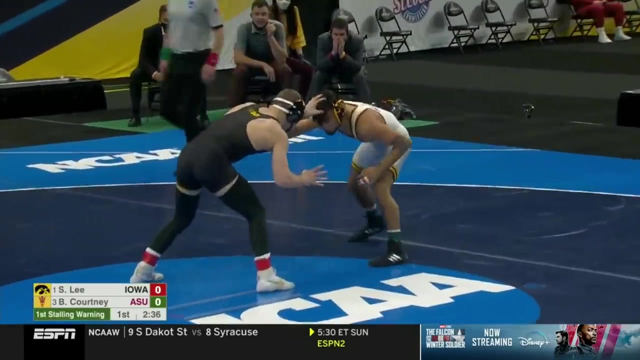 as well. one high school, two finalists, with Kemmerer and Lee Spencer Lee, the reigning Hodge Trophy winner. giving you an idea of just how dominant he's been: He won 52 of 57 first-place votes, the largest margin in the history of the award. 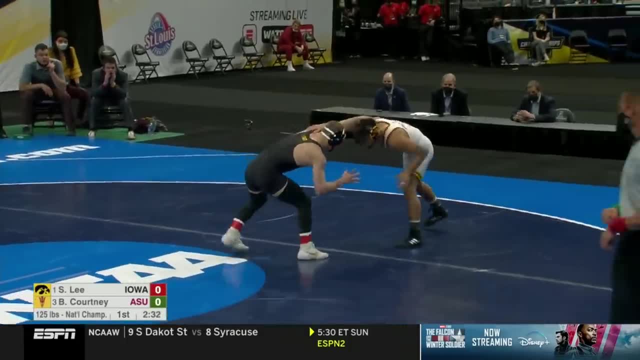 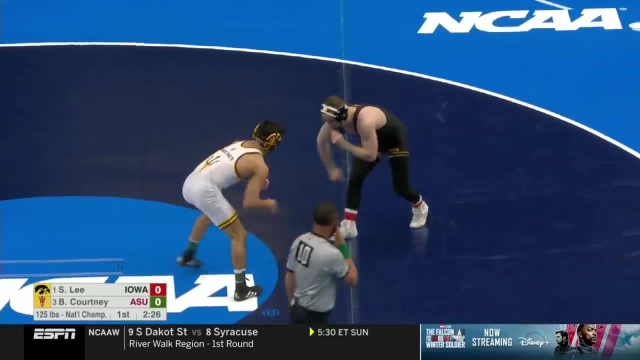 And that's a bigger margin than when Joe Burrow won the Heisman at LSU And he's been one of the most significant Iowa wrestlers in program history. I think that he's you know. you always want to take advantage of it. 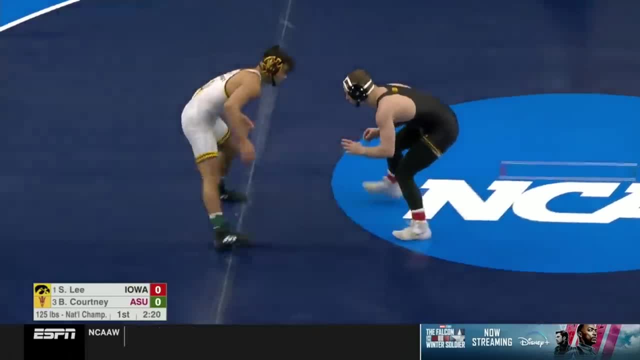 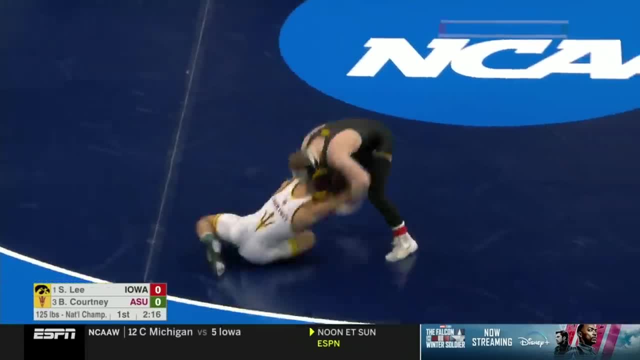 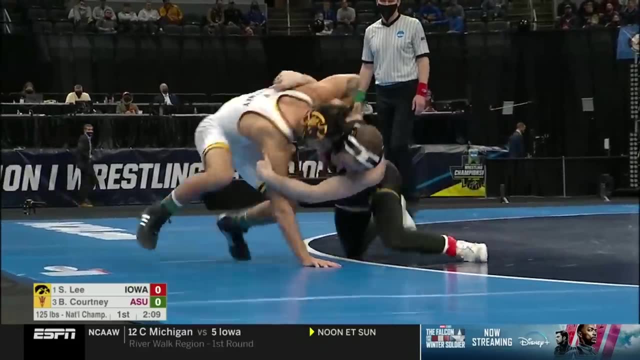 Leadership. That's exactly what Tom Brantz has done: leadership, leadership, And just you know the guy who's been, you know can you just tell the affection that he has for his teammates, his coaches, is everything you want to have in a program leader. 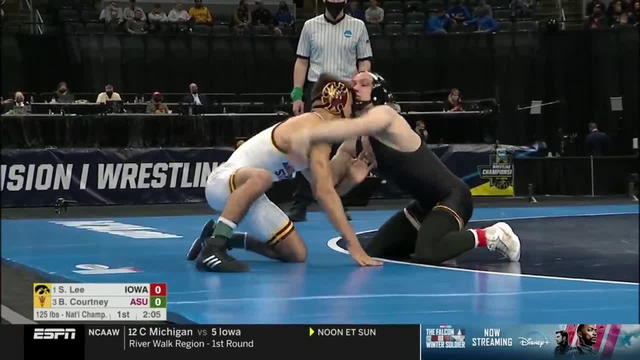 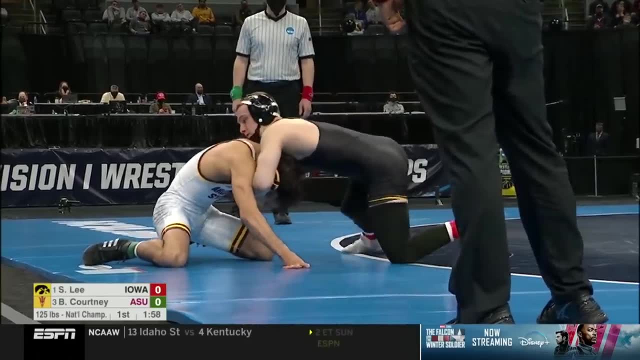 is everything you want to have in a program leader. is everything you want to have in a program leader. Rattle in here, Rattle in here. Not only a Hodge Trophy, but the Sullivan Award winner as the nation's best athlete. 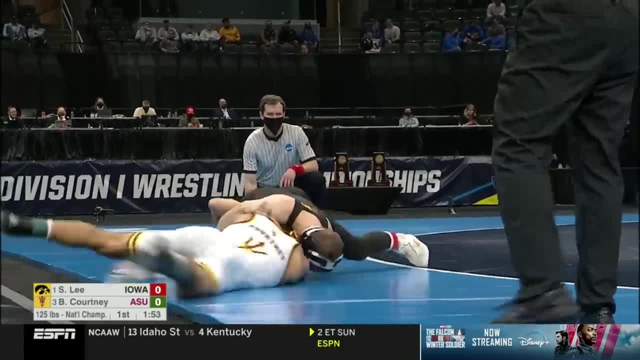 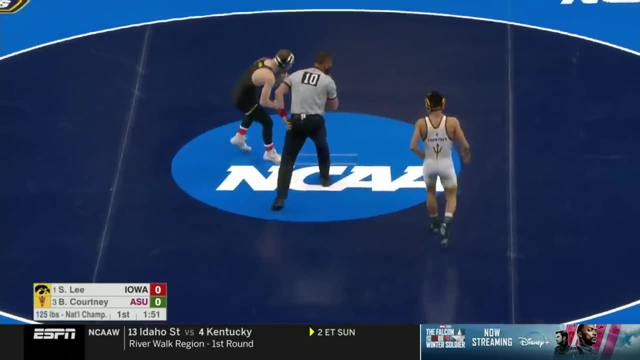 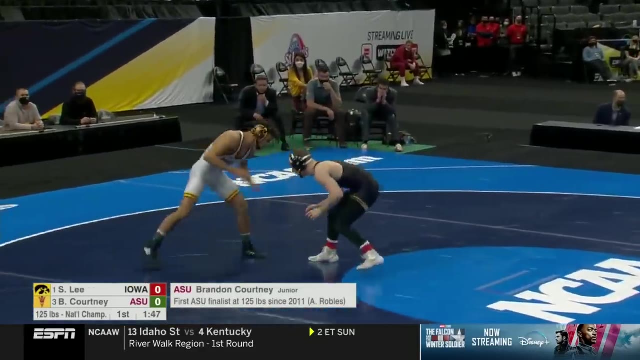 as the nation's best athlete. Whip over their situation. Whip over their situation. Courtney's going to go off and Courtney had to do is what he's doing right now is creating a lot of motion. He saw that nice little collar tie stamp. He was able to hit on Lee. Can he continue to dance and possibly get his attacks off from distance? And Lee stalks him. takes a shot of his own. 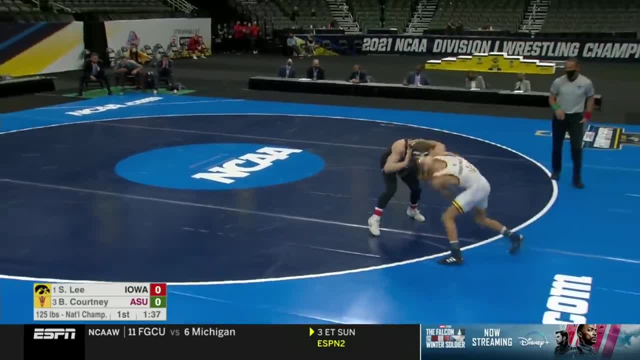 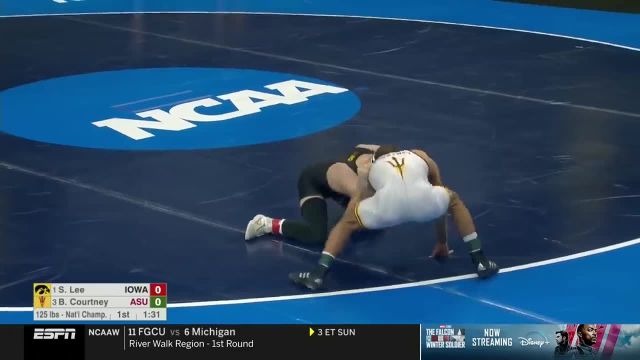 He needs to break free The boxer. that lets him get a little more space to hook from him. now is in a rip over situation. Lee is really just trying to go ahead and clean down. get to a leg, Seems like when he don't, you're always off the mat. 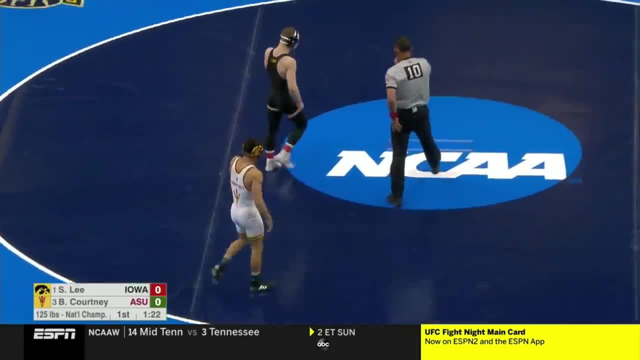 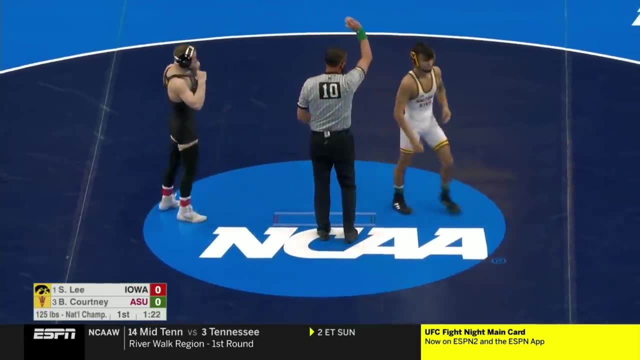 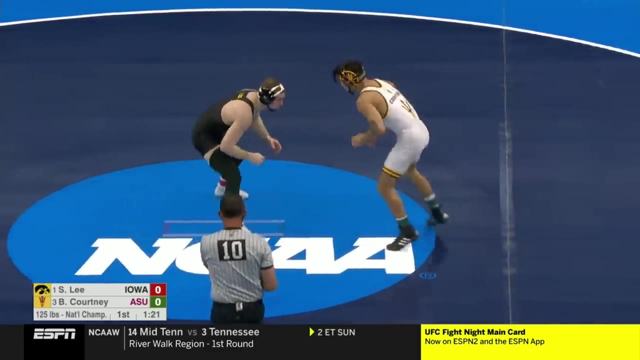 Courtney and Lee go out. Courtney, the red shirt junior, on an 18 match winning streak. Arizona State has had nine wrestlers win an NCAA championship. The most recent was Zahid Valencia at the last championship contested back in 2019.. And a second false start there on Courtney's One more, and that would be a point for Lee. 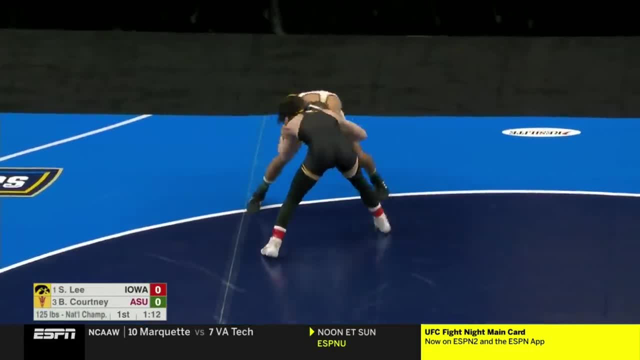 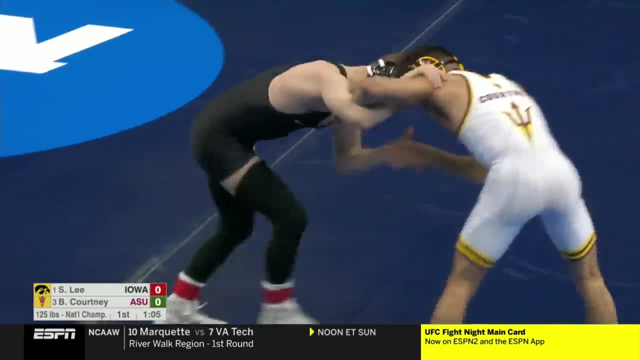 You notice Lee has both knee pads on. You just wonder what that means. You know he's had one knee with a lot of trouble and surgery. Whether that means both are hurt or not, it doesn't matter. And what then doesn't matter is the 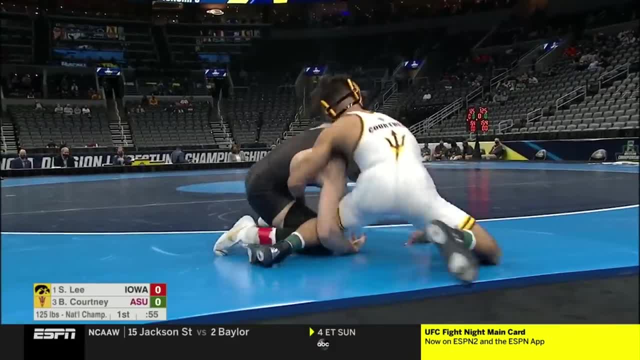 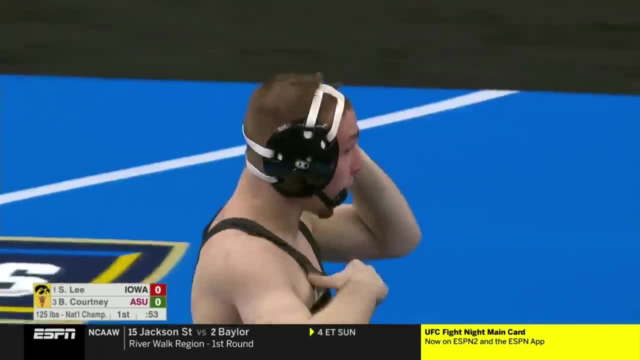 It's not a question. Lee has been so dominant in his career. It certainly hasn't affected his performance, The tight matches. he hasn't had tight matches, but the matches he's been in really have been, because the other guys, I think, have improved. 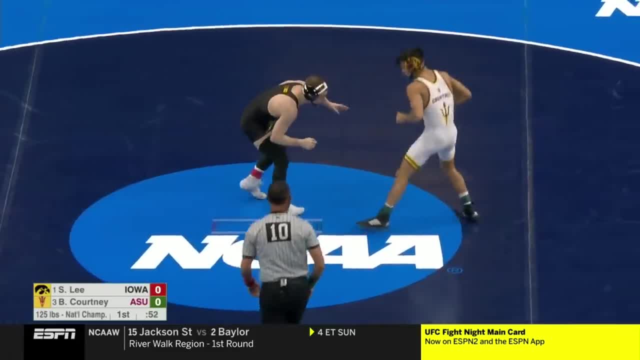 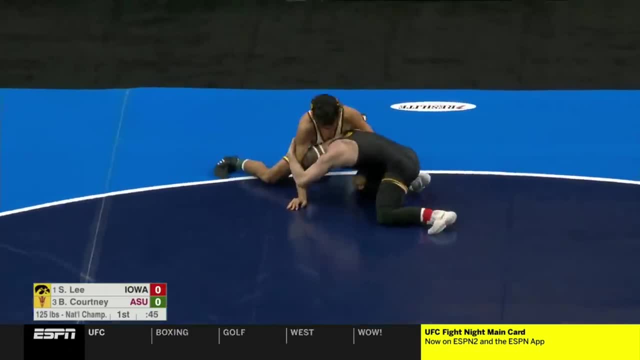 Stay in your work. Stay in your work. The toughest wrestler in the top position- And I'm sure that Courtney doesn't want he- will not choose the down position. He'll either. defer Exactly: This is as long a time as Lee spins on his feet. 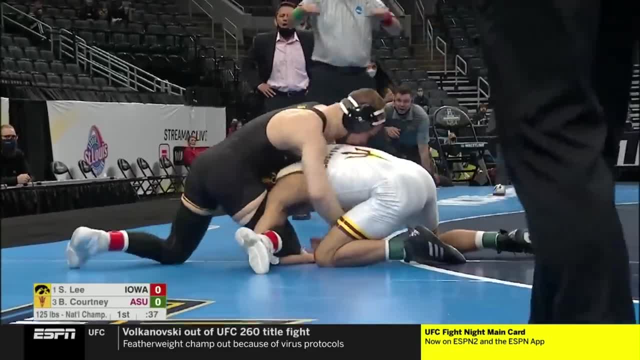 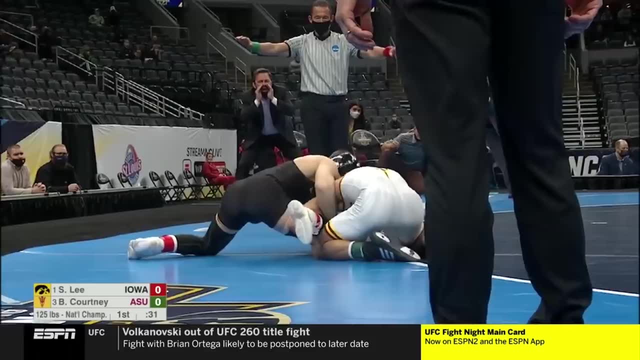 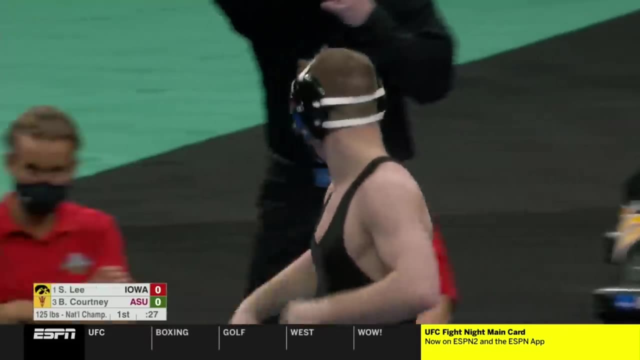 85% of every match in them. you know a shot by Courtney on the edge, No points awarded. The Arizona State corner Zeke Jones wanted it. They go out again 27 seconds left in the first. Like I was saying, Spencer Lee spends 85% of his time on the mat on top. 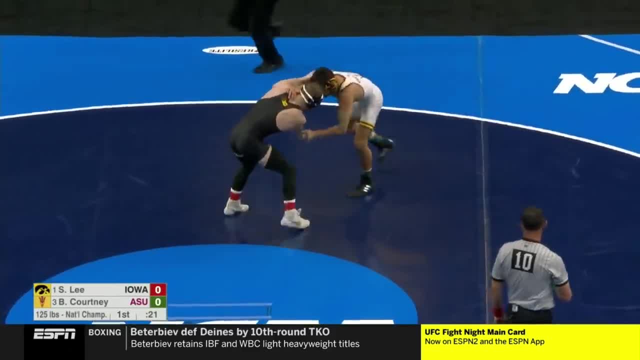 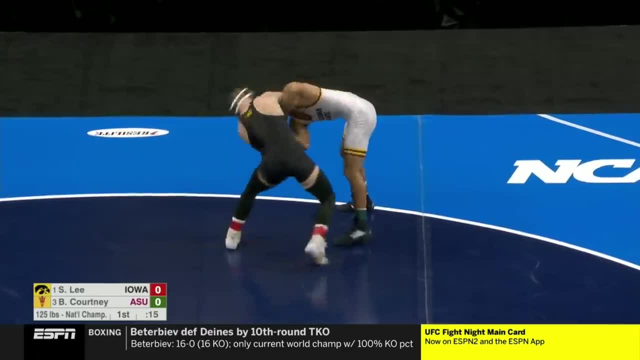 And right now we're almost finishing an entire first period without getting there where he is most comfortable And lethal. Mainly been due to Courtney's footwork, He's been able to go ahead and hit the edge, And it's the first time that Lee has not been able to get that penetration step like you're talking about. 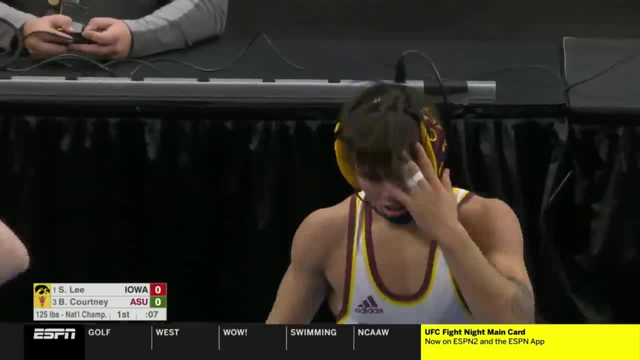 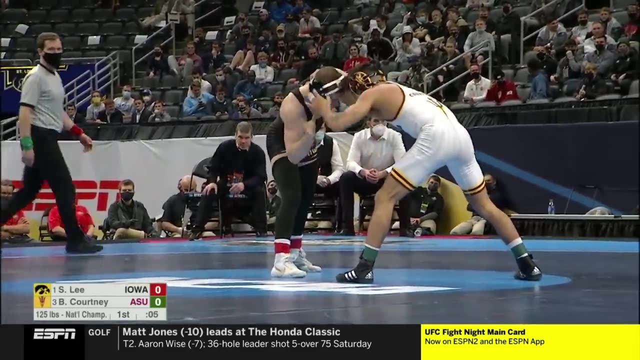 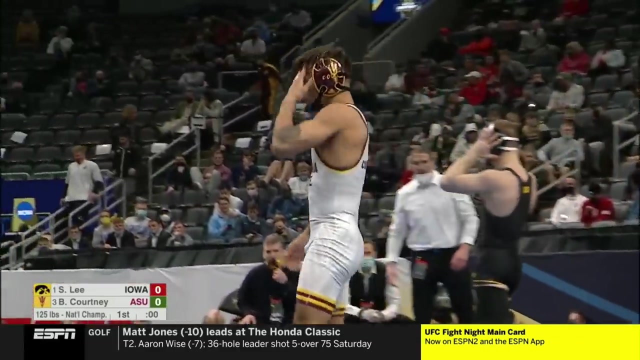 I wonder what the Mentioning here Tim has some substance to it. Of course. we've seen the additional knee sleeve, So it's a scoreless first, Surprising at all. Yes, I mean, this is the great strategy, though. 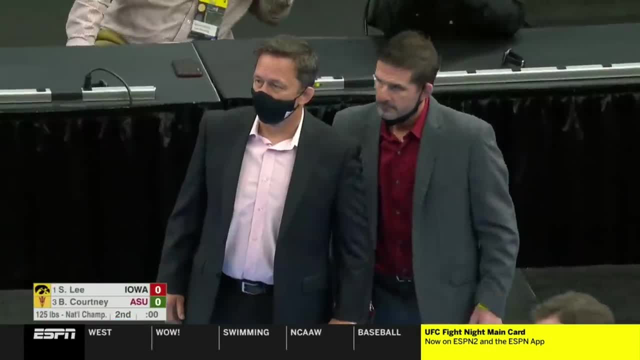 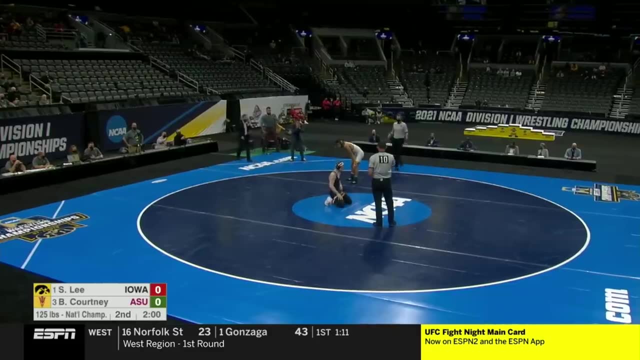 And, as Jim said, the footwork of Courtney. But you've got to try to take the lead at deep waters to dark waters and keep the score close. And so far, so good. Hey, here we go, Green, get in there. Two cautions: 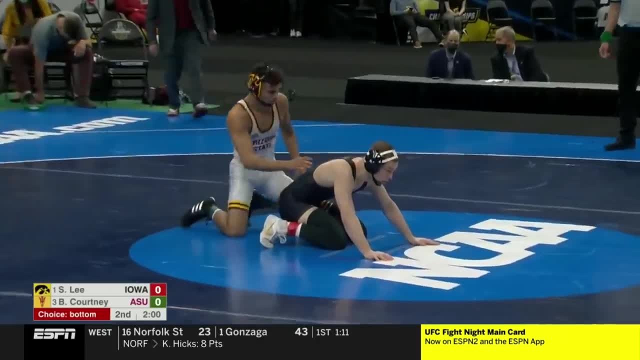 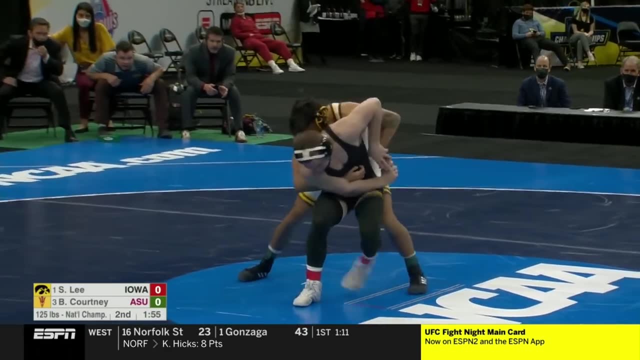 Hey Green, you've got two cautions. Lee, this year, Get on The number one, The number one seed in back-to-back years, The first 125-pounder to do it in consecutive years since 2001 and 2002.. 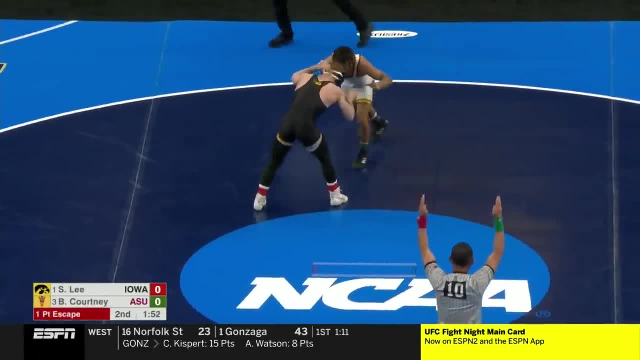 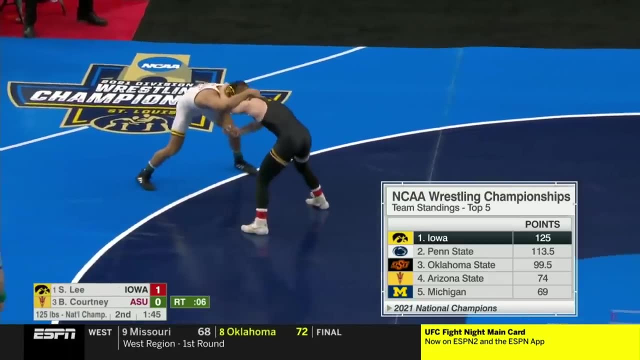 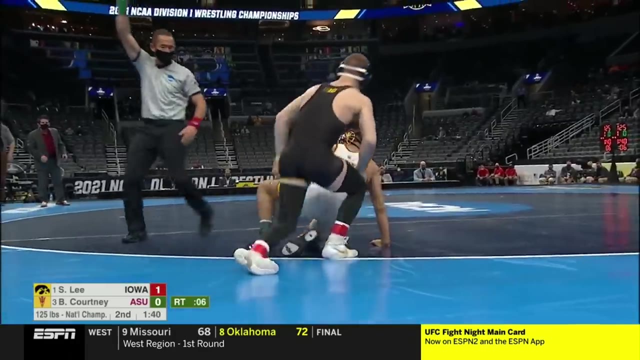 Steven Abbas at Fresno State. Quick escape by Lee. Final match of the night. Iowa coming into this championship round locked up in the 2021 National Championship, Their 24th, second, most all-time. There is a warning. Stay in here. 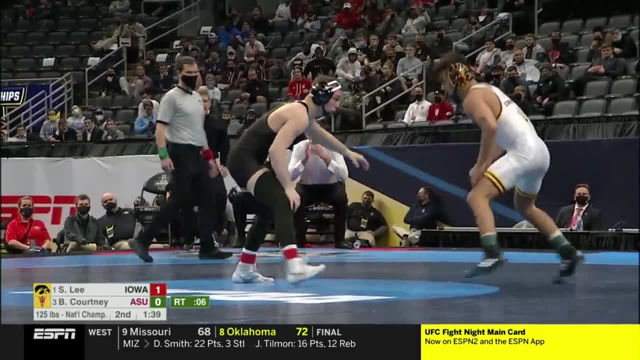 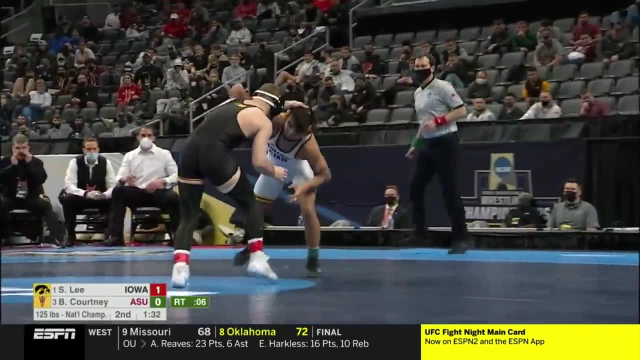 On Courtney: Yeah, I think Spencer's done a nice job of even though they have all that motion out in front of you. he's taken territory, gotten to the edge. He hasn't allowed Courtney to get to his corner, Got shots off at the edge of the mat. 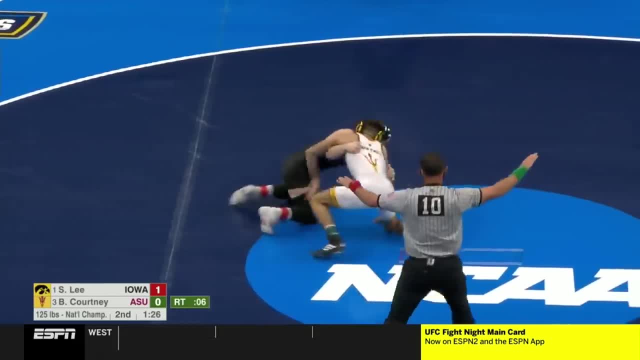 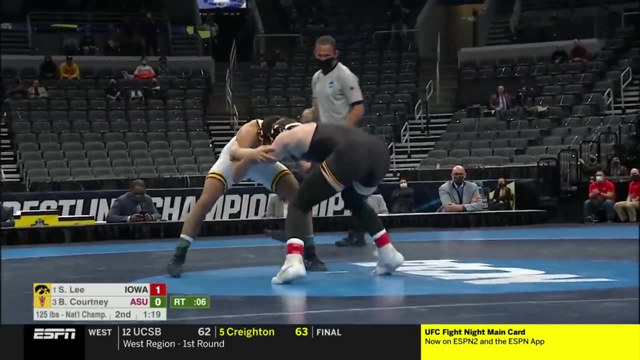 If a guy's going to play the edge like this, he's going to get called. Courtney did a nice job of bull rushing in there but hanging on with a little underhook there. This is the tightest look that Lee had on Courtney. 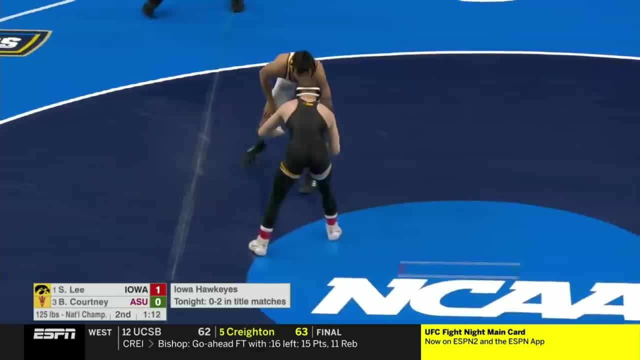 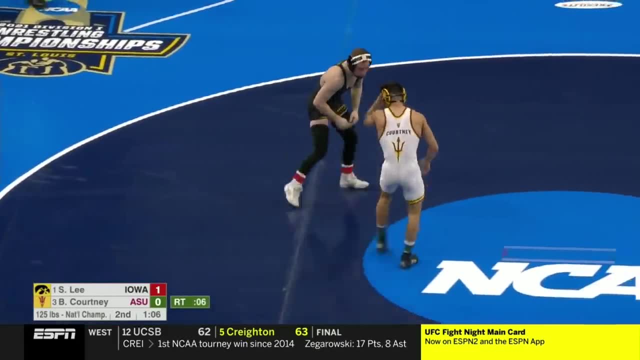 He didn't follow through with it And Lee pound for pound as strong as any wrestler out there. But that poundage is his entire body and it comes from the plant of a foot as much as it does that underhook, And so you just wonder if that plant is affected. 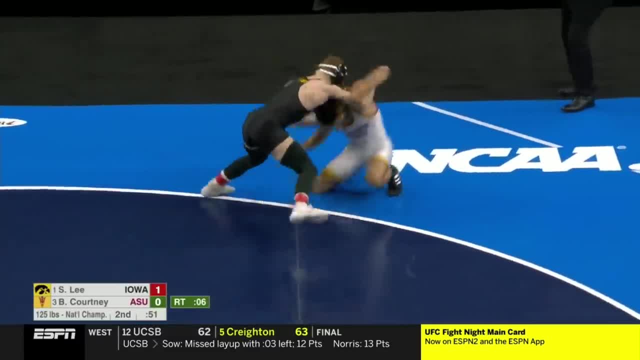 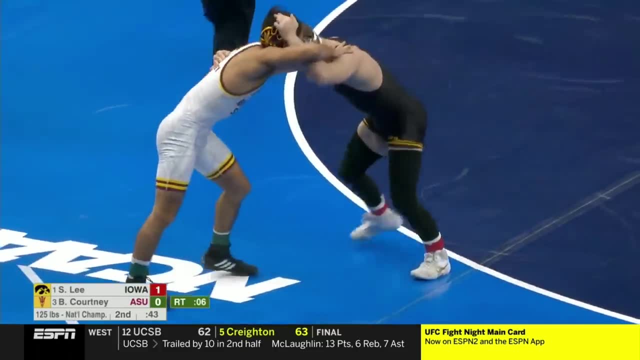 A little drop down there. Now he's going to The other thing too. Tim is what's happening here. He's got that underhook on the right-hand side. but notice how Courtney Back up- Not necessarily, Not necessarily in this situation, but he's quickly getting one leg up to fend off that little rip-over attempt right there. 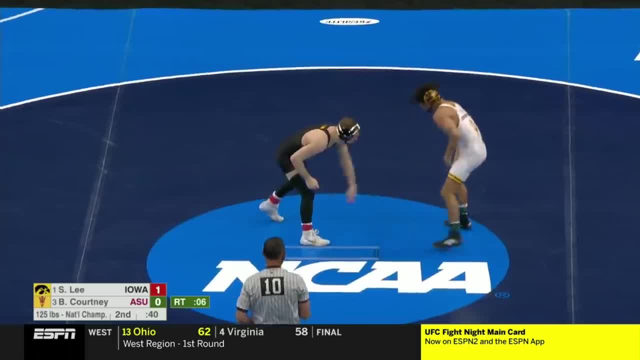 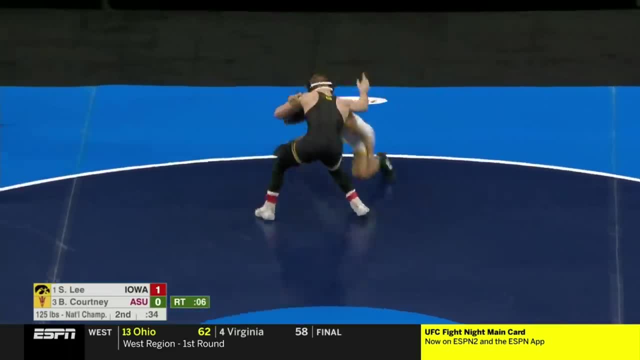 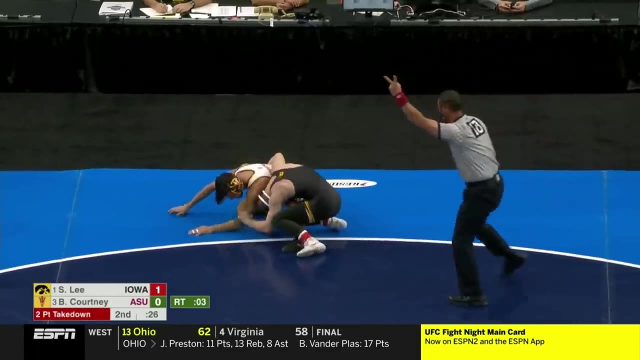 He's got his right leg up allows him to come to his feet. Yeah, Given the dominance of Lee this year, bonus points in every match. rare to see a 1-0 score here this late. He gets two Tremendous job right there at the edge with the two points. 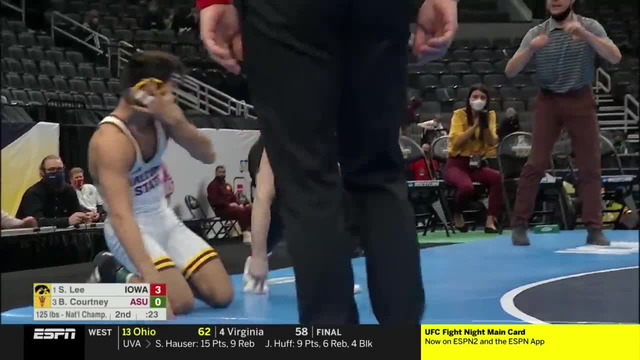 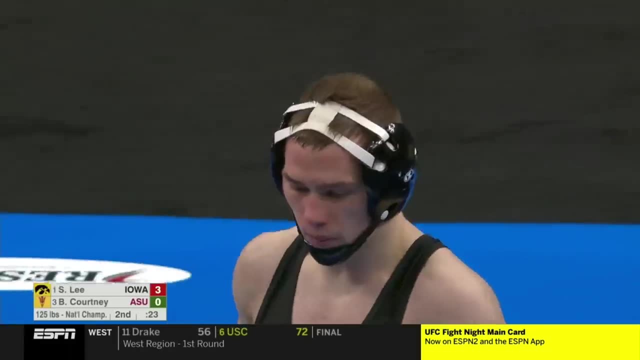 Now on top. Yeah, he pushed him to the edge, made Courtney take that kind of wild waving that shot and was able to drag right around and anticipated that shot by Courtney and he's been rewarded- Wait for me. And with all that pushing and moving, he forced his opponent to go ahead and take a bad shot. 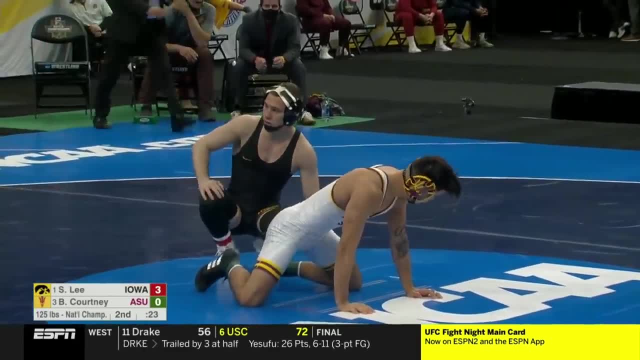 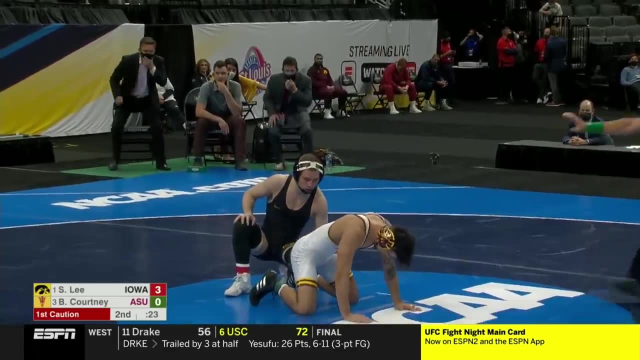 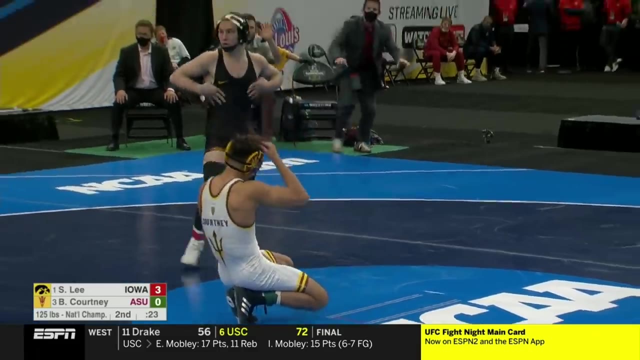 Top man: Okay, don't roll. Don't roll here. Two green, one red- Yep, Okay, wait for me, Get on Set. Set. Top man Set. There's his third. I saw two from the standing position and you heard the official warning. 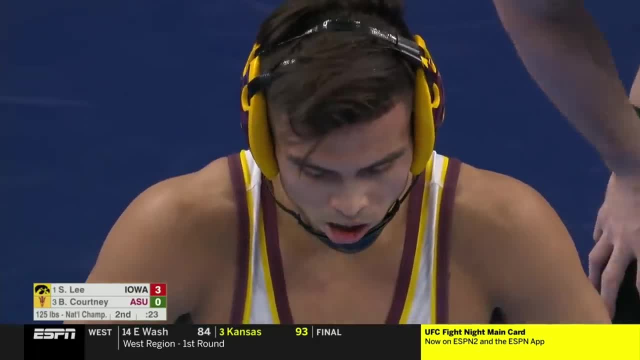 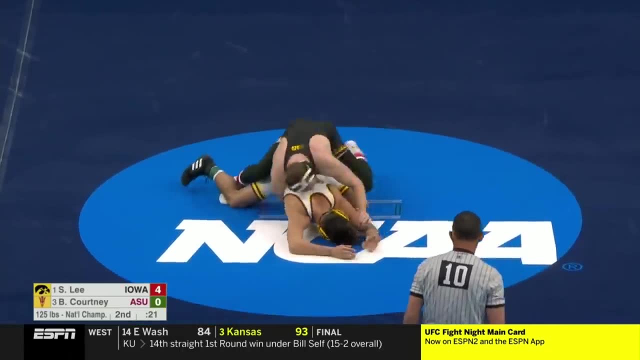 Starting at the second period, you have two cautions. Wait for me, Get set, please. So 4-0 Lee. So he goes on top here. This will be the first riding time of the match And it's the longest we've gone in a Lee match. 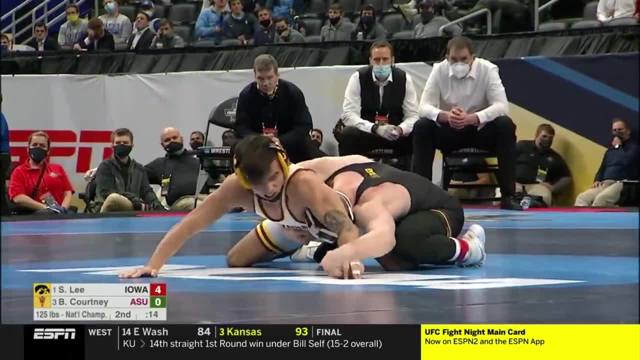 We're not talking about his reinforced bar tilts and how tough he is on the mat Head lever as he does it. Nice, Nice job of bringing it back there to try to trap that wrist Gets the wrist and then Or the bar. 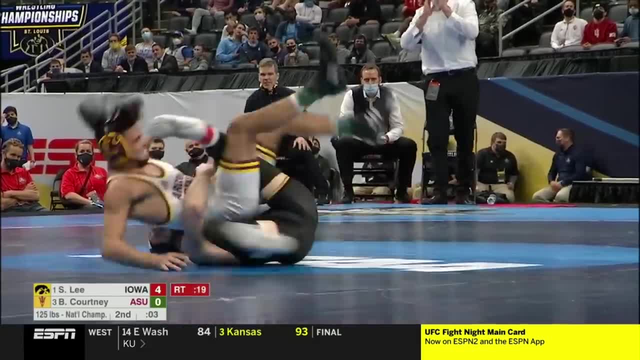 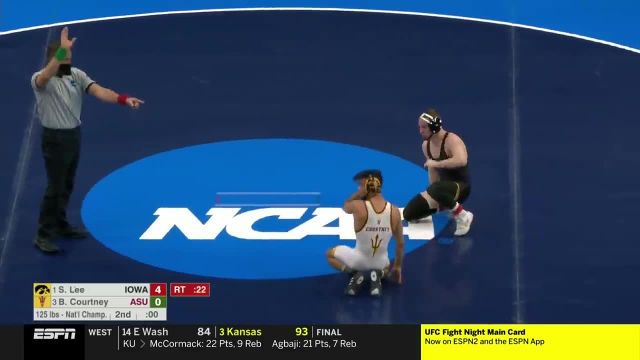 Watch the battle. right now He's hunting for those tape fingers. right there He's grabbed one and now he's going to go right into his tilt. He got one swipe and then reached the end of the second period. Green choice. 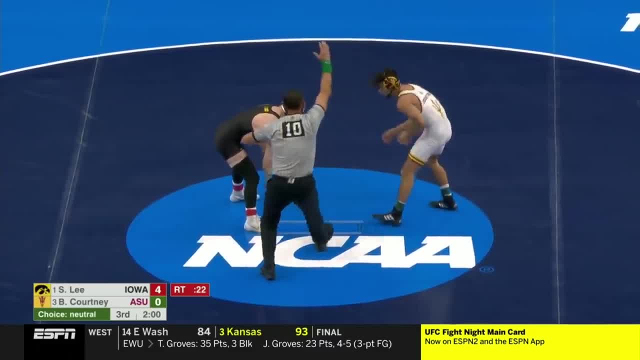 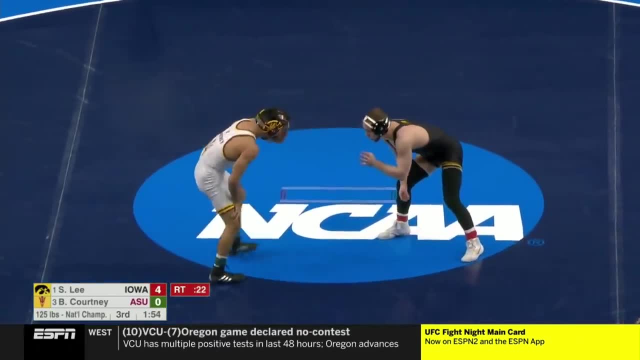 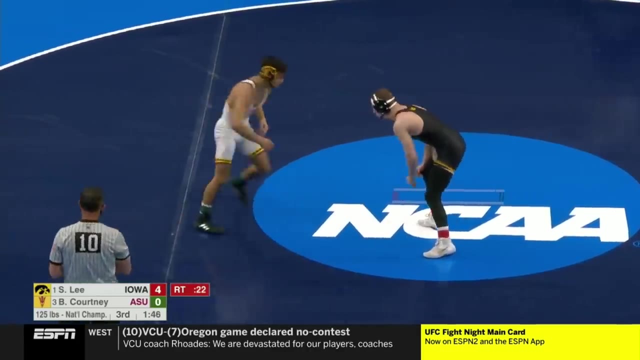 Courtney chooses neutral, Here we go, Get it on, Here we go. One period away from a third national championship for Spencer Lee And if you're Courtney, you're down by. you know four points. Got to create enough activity. you know your strategy of kind of keeping it close has worked. 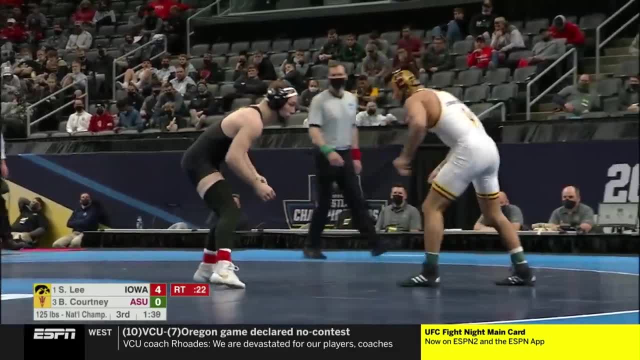 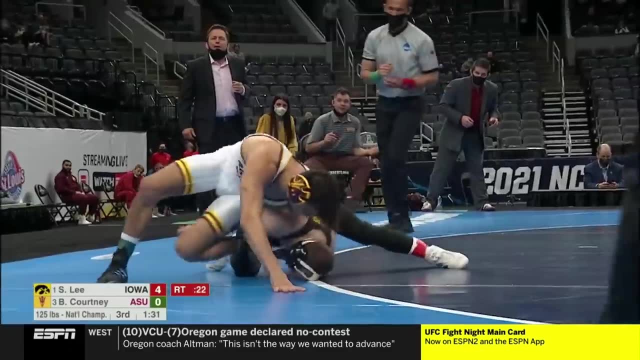 at least to this point, when you're, you know, only four points down, But you got to start taking shots in this direction there, And that's going to make it a little bit easier for Lee to score. Nice slipping, Very nice job. 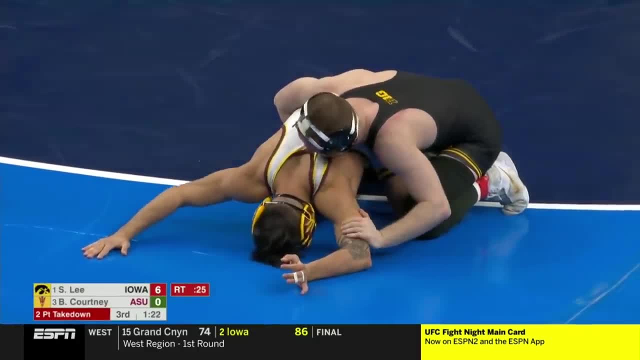 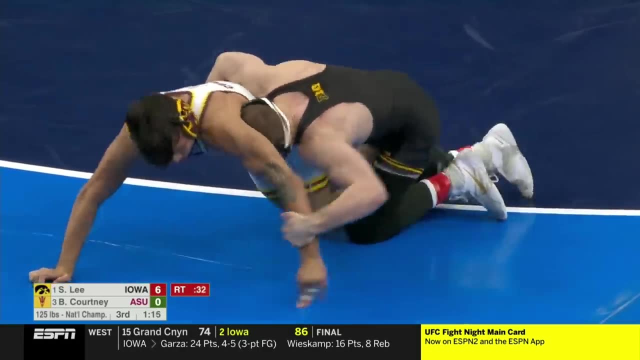 Limping that arm coming around covering the legs and the hip for two at the edge. Lee's advantage now 6-0, trying to become Iowa's seventh three-time champ in a group that includes Banning Brands, Barry Davis, Lincoln McIlravey. 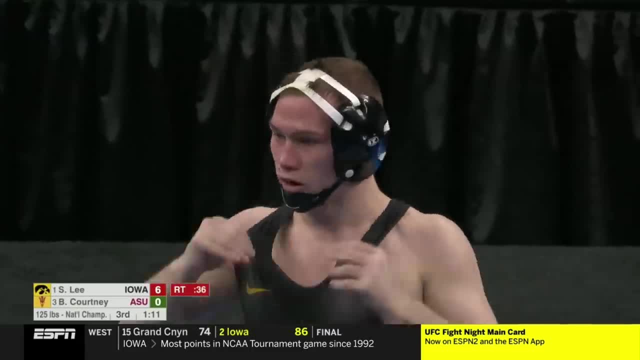 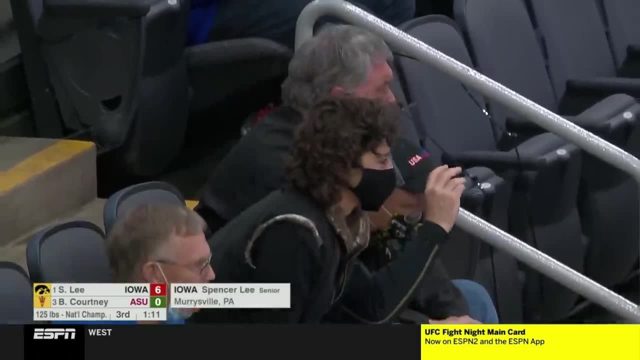 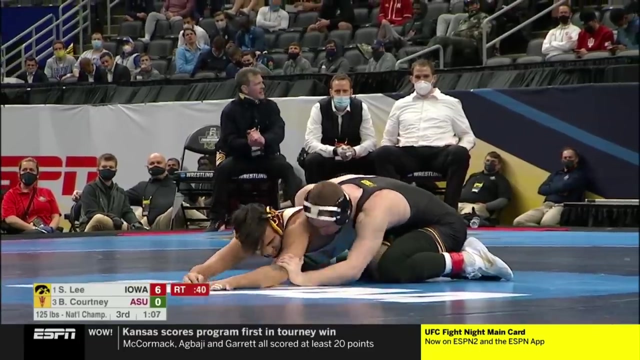 Joe Williams and Jim Zaleski. He grew up in Pennsylvania. The choice really came down to Penn State or Iowa, And as he grew up watching videos of Iowa wrestling, he realized that he was going to be a Hawkeye. That was part of the draw, along with Terry Brands. 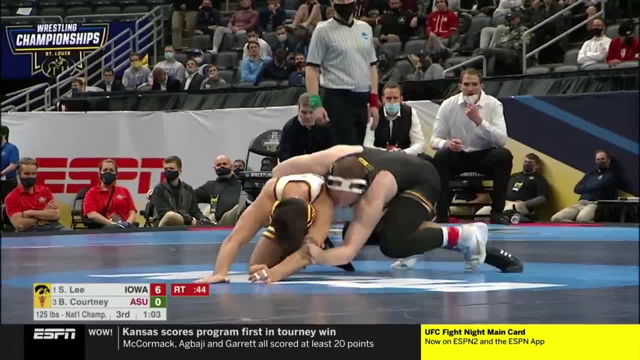 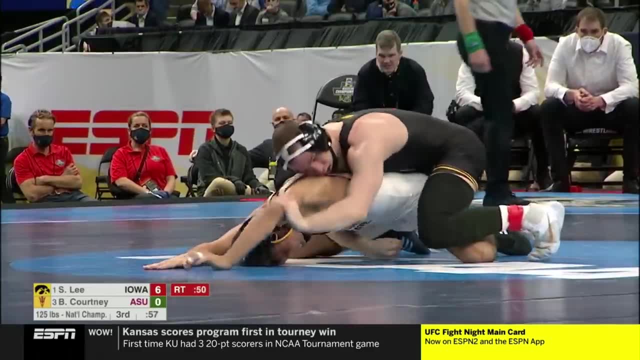 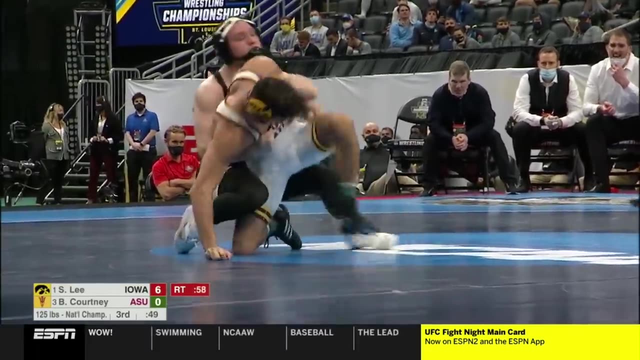 made him want to be a Hawkeye. He's been working hard with his head and his armpit right there trying to capture that wrist Right there. he's got it captured. now Watch him work that up into that bar arm right there, with the left arm coming up in. 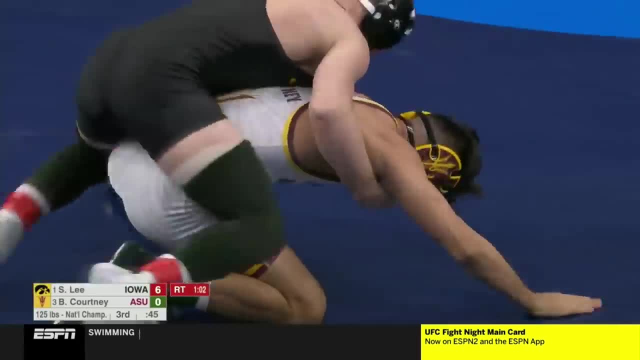 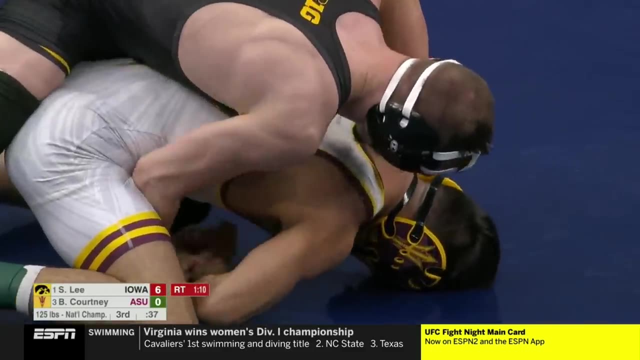 Now he's going to actually work the tilt without actually And he gets that bar arm Below the elbow there and it makes it so that Courtney cannot really use his left arm there for any kind of power to bring it down. There's a big debate out there going on right now whether you know. 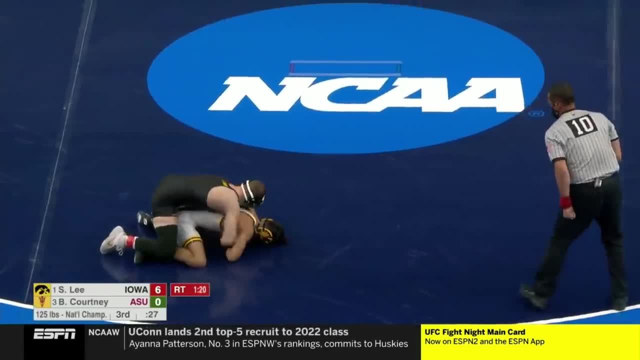 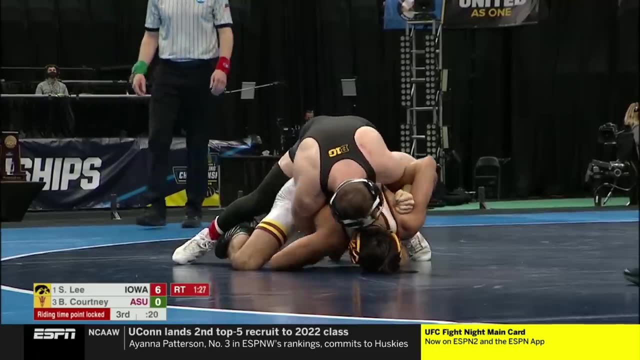 I'm sure the officials are wondering, but it's certainly legal right now. But I'm sure the officials have heard whether this technique is legal or not, but it's irrelevant right now. This is what this guy's doing to turn guys effectively. 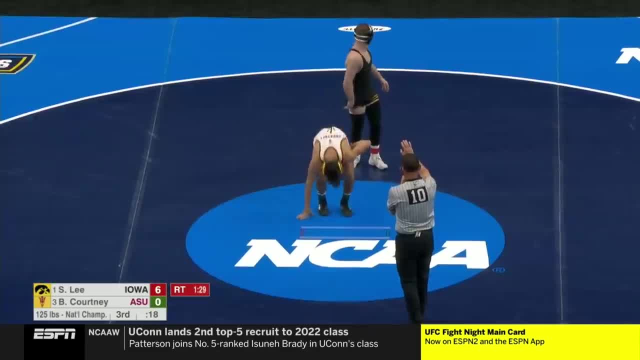 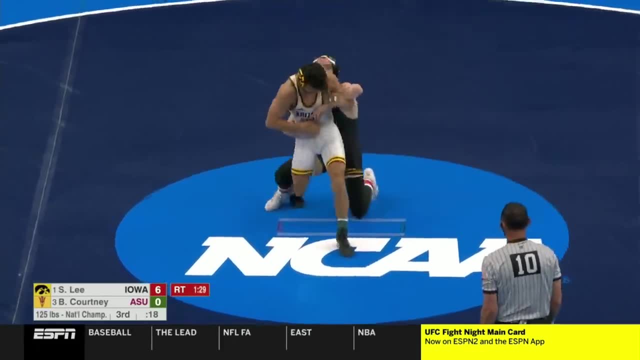 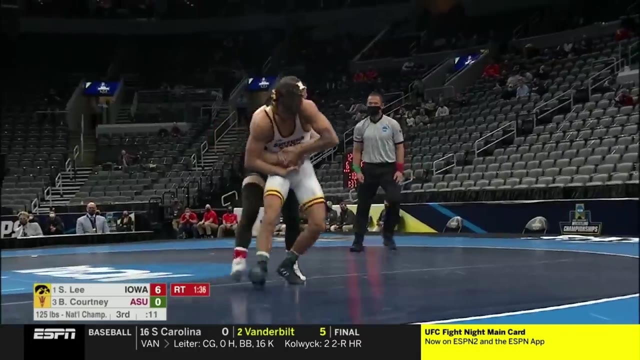 Working pretty well for it. Wait for me. Red Set cover. Yeah, you hear the No, you're good Officials. during that sequence, there were always talking about keep it legal, keep it legal. Well, that tells you that they're onto something there. 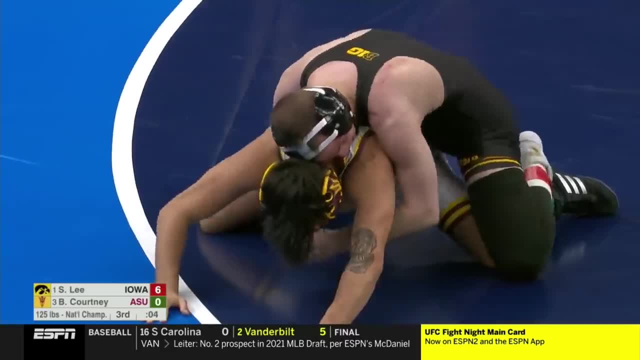 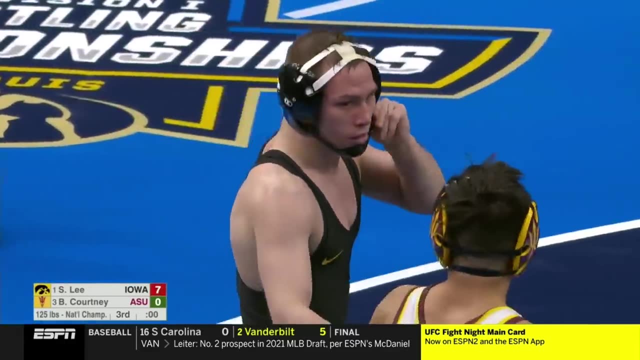 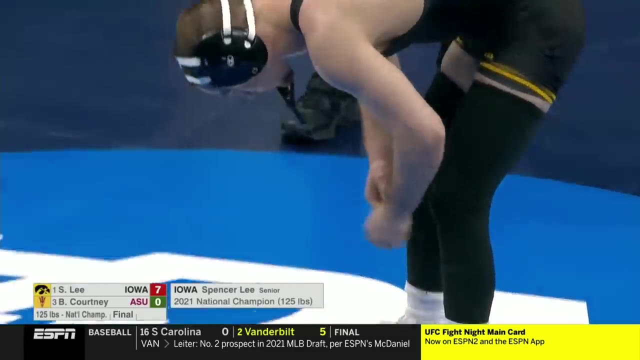 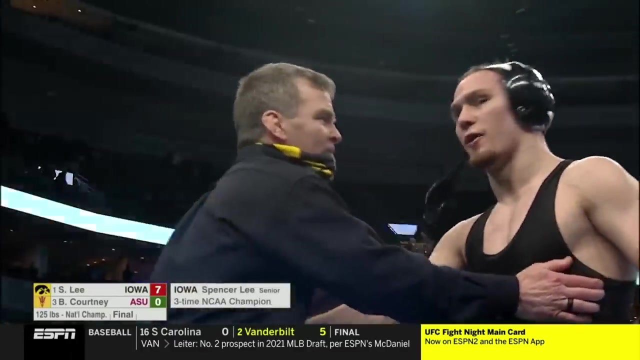 But Lee has done that. He's going to win another national championship. The Iowa Hawkeyes the team champions and Spencer Lee is Iowa's seventh three-time national champ- The only time all year he didn't win with bonus points and it didn't matter now. 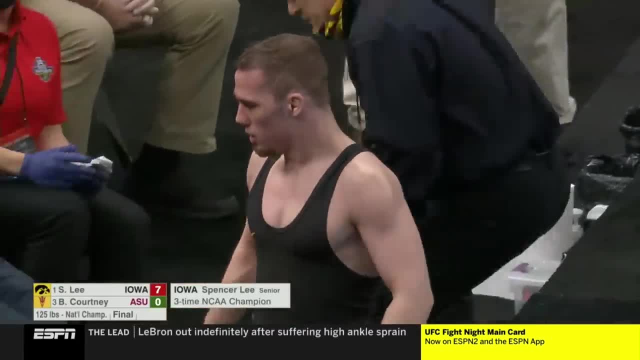 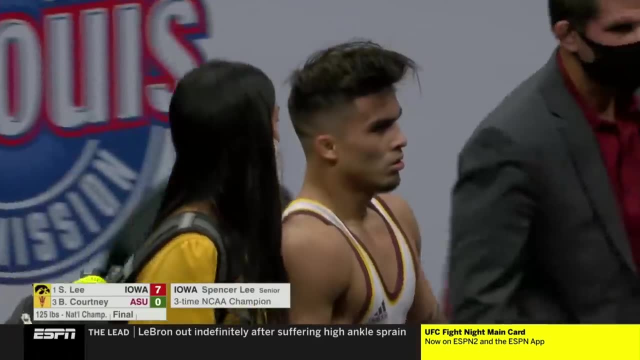 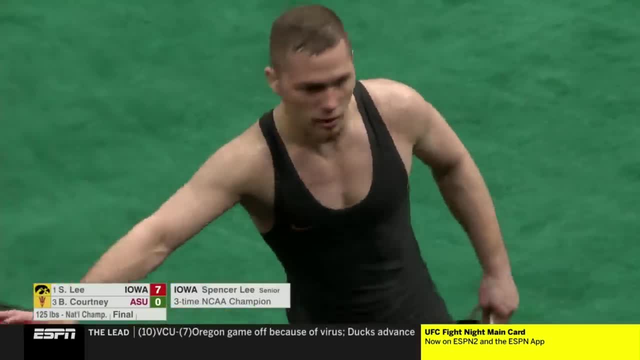 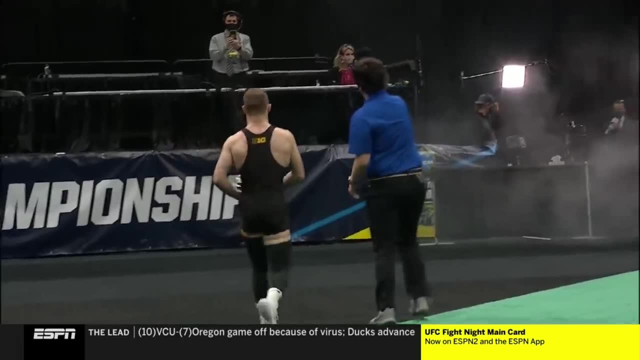 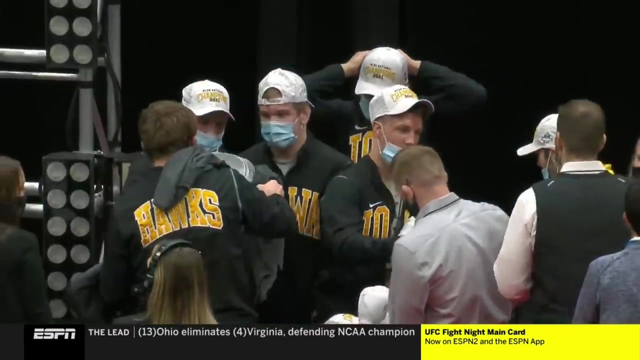 He's going to win The humble hero for the Iowa Hawkeyes. They gave him the name Yoda this year because he can just do things that they say are a bit unnatural. They're both a little bit short but large in stature, Quinn. 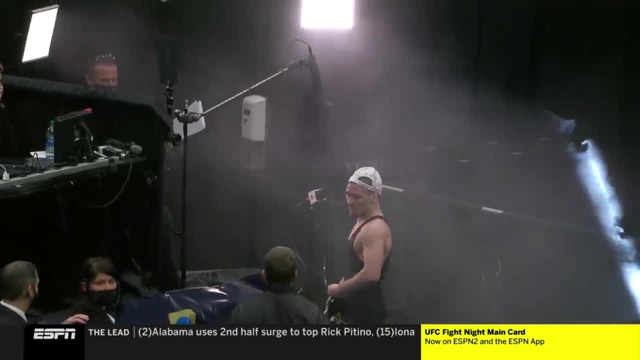 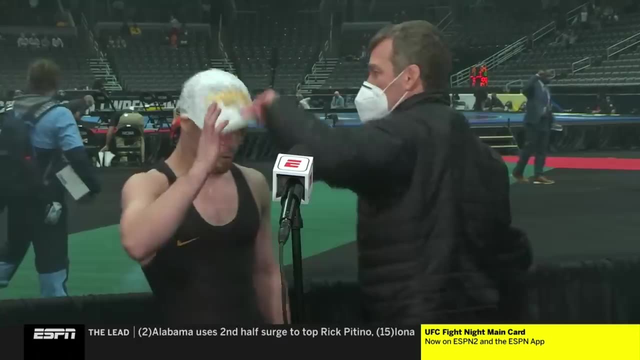 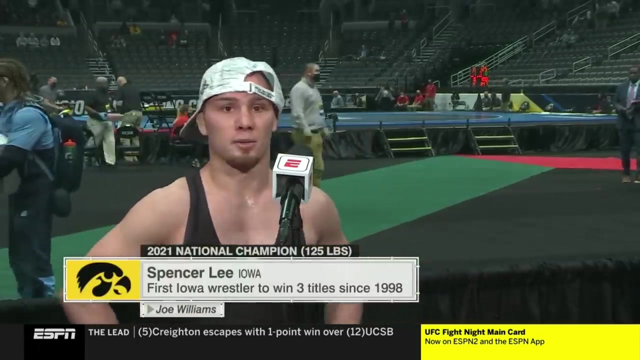 Humble example and team leader: Patience. A hug from Tom, I believe, even with a mask on Tough to tell Spencer you said: this is what I live for, This is what I was born to do. What's your reaction to winning this third championship? 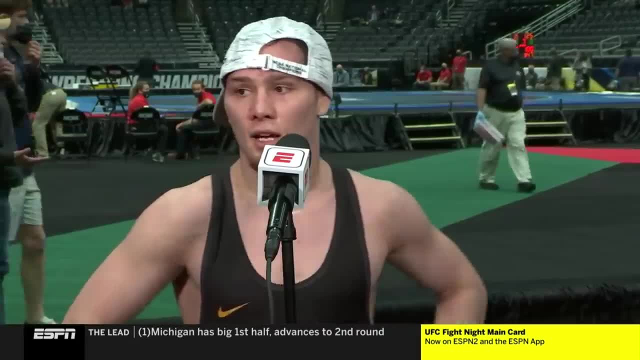 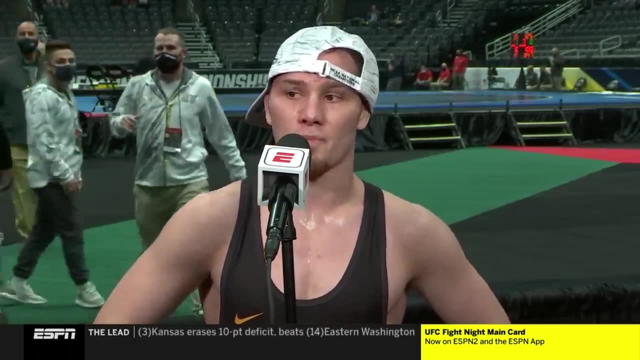 I went through a lot. This is definitely my toughest. Yeah, I'm battling a lot of things. Yeah, you insinuated that yesterday. What are you battling and what's the adversity been like? Well, I mean, Eight days ago I tore my ACL in my other knee. 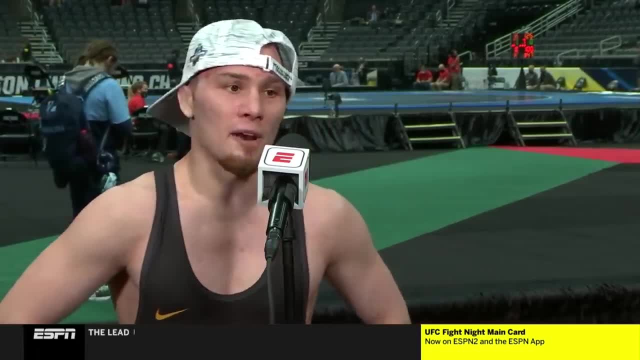 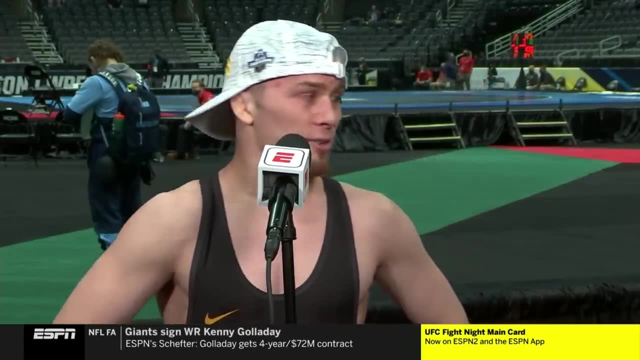 I'm wrestling with no ACLs and you know whatever, man, I didn't want to tell anyone because F excuses- Excuses are for wusses- And you know what. That was a tough turn for me. I could barely wrestle. 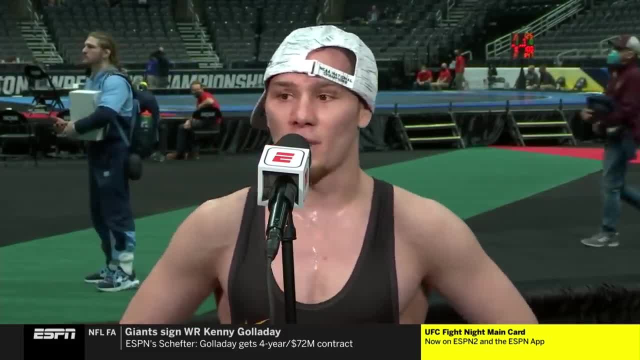 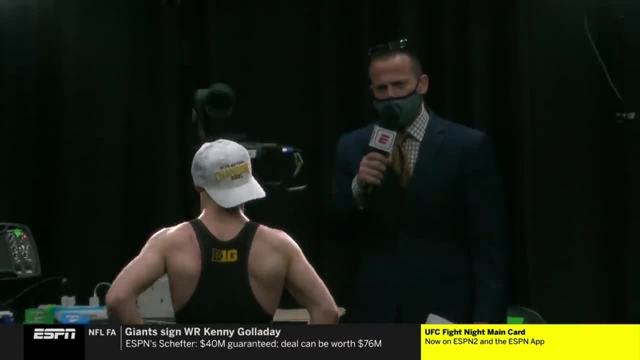 I could barely shoot, I can't sprawl, But you know what? I believed in my coaching staff and everyone that believed in me. and here I am. so there you guys go. How did you handle the self-doubt? Well, I mean, there was no doubt.